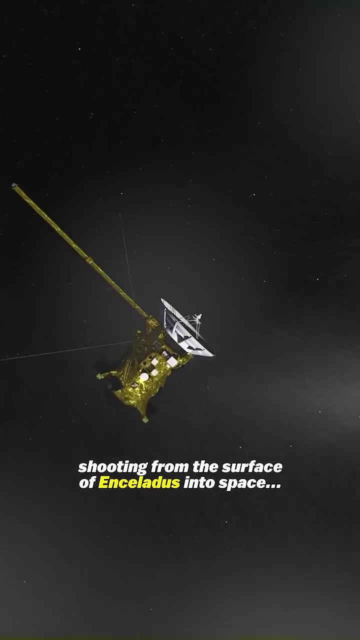 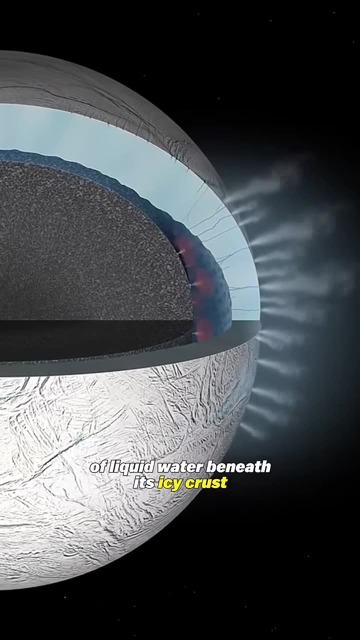 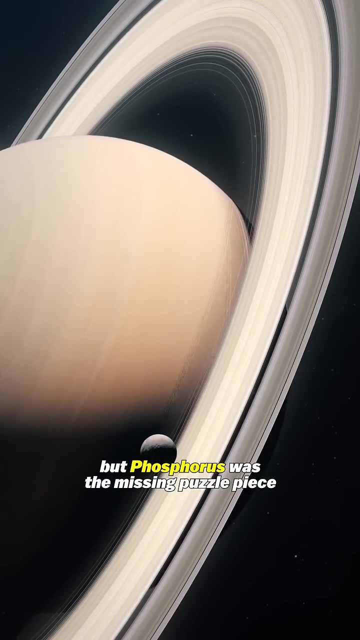 evidence of phosphorus in the water: geysers shooting from the surface of Enceladus into space. Enceladus has this huge ocean of liquid water beneath its icy crust, and we previously found the five other key ingredients for life in the ocean, but phosphorus was the missing. 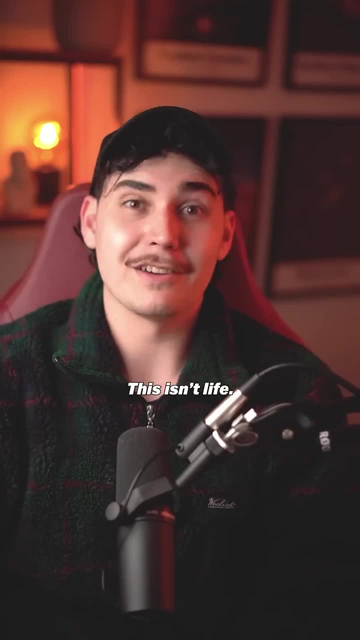 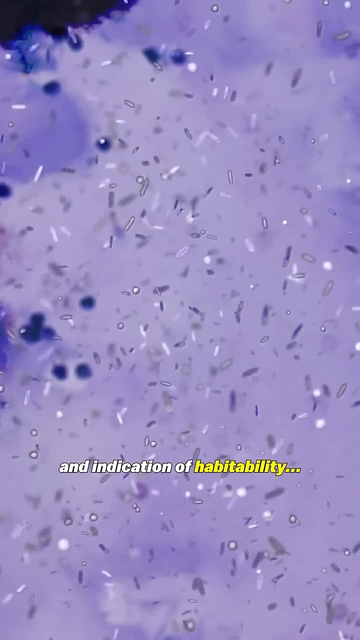 puzzle piece. Now let's be clear: this isn't life. they haven't found aliens, but this is a really exciting discovery and indication of habitability. So if we do find life outside of Earth soon, Saturn's moon could very well be their home.